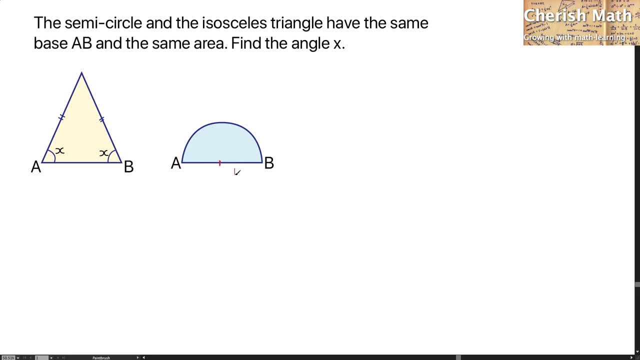 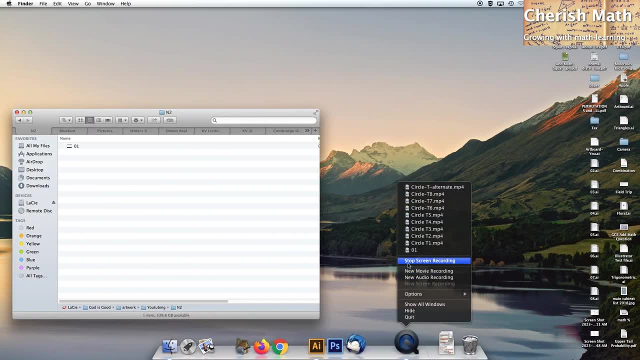 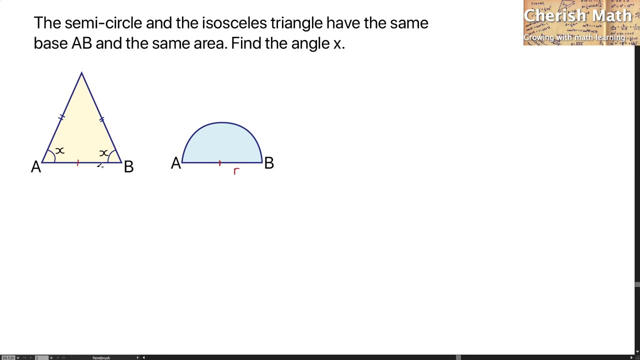 semicircle is AB. Half of it is the radius that I'm going to label with the letter R For the triangle on the left-hand side. half of this length of AB is the same as the radius of the semicircle, which is I'm going to label here as R as well, And I'm going to highlight the height of. 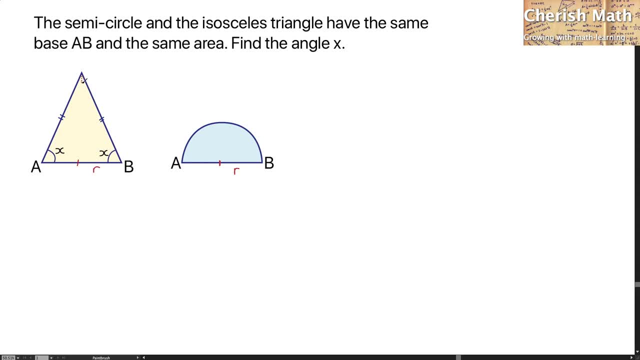 this triangle with the letter H. I'm going to work out what is the area of this triangle by using the formula of one half multiplied by the radius of the semicircle. So I'm going to use the formula of the base width multiplied by the height as the formula of the area of triangle. 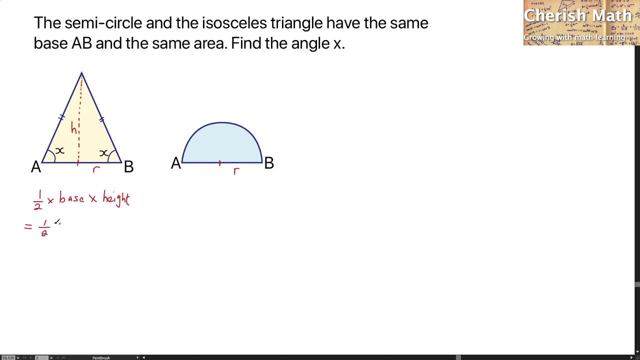 And the working here is one half multiplied by the base width is AB, which is twice of the R multiplied by the height that I've labeled here with the letter H. So I will be getting R H As the area of this triangle, And now I'm going to work out what is the area of the semicircle. 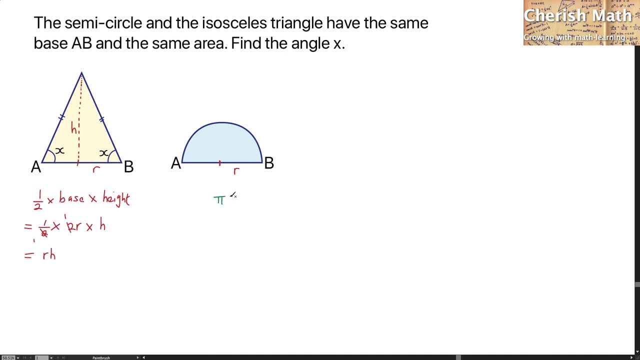 The area of the semicircle is pi R square. Since this is semicircle, I have to multiply by one half and that's the area of the semicircle. I know that the area of the semicircle and the area of 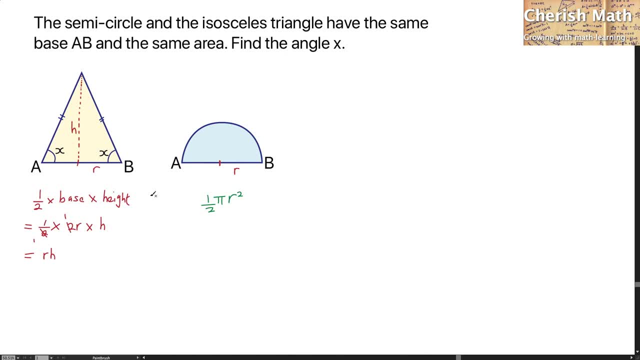 this triangle is the same. That would be. I just need to equate it directly with R H to one half pi R square. The equation here would be R H equal one half pi R square. We need to simplify your thing here now. 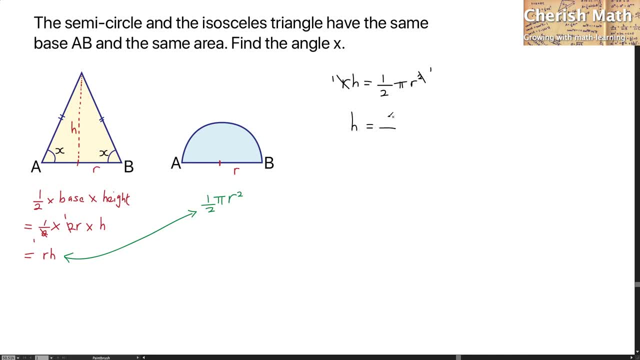 So H is simply equal to one half pi R. I'm now almost at the final step in solving the problem. By looking at this triangle, we know that here is actually going to form, with 90 degrees, or the right angle, The angle of the X. I can find it by simply using tangent X.